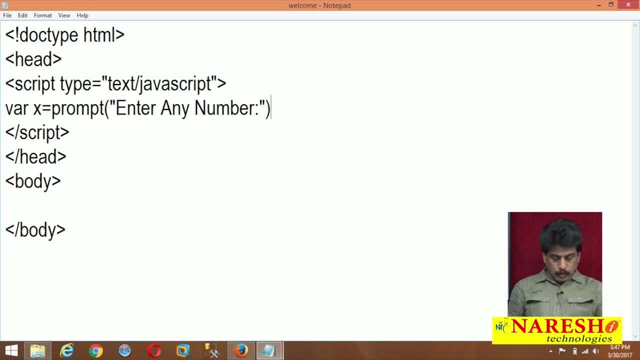 Any number you want it by default number also you can take, And for that purpose view the syntax of the prompt And now I am providing: by default number is 5.. So x is equal to Now. if x greater than, for example, 100, I provided then alert user. 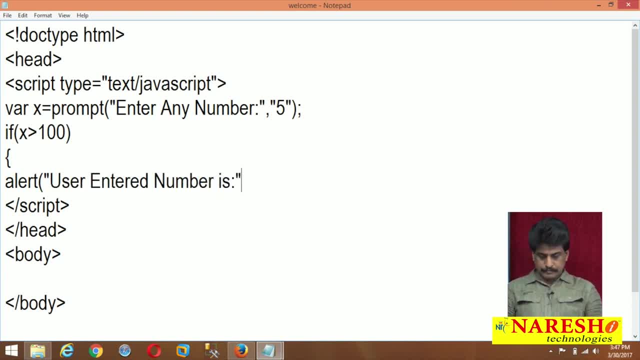 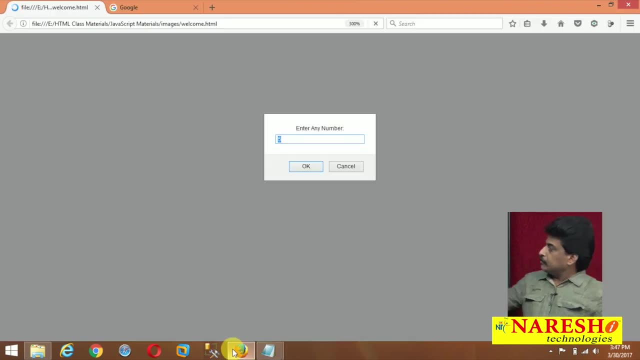 Entered number is plus x. That is all I am not writing. body section does not require That is the head part. Come to browser refresh. By default number 5 available. For example, I am entering 101, greater than 100. Then displaying user entered number is 101 because 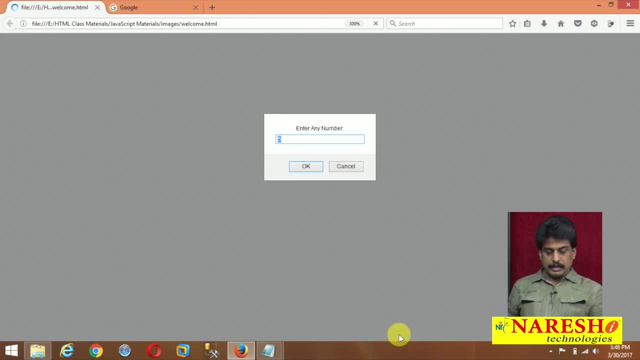 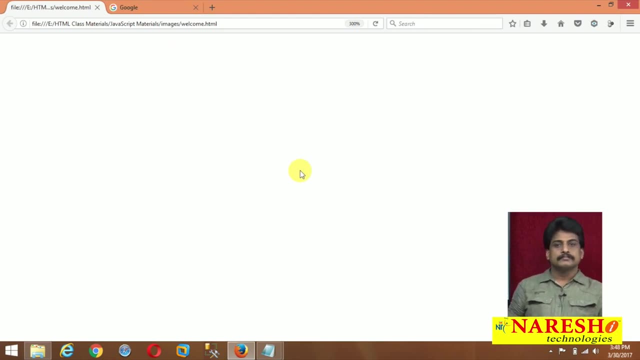 true. Now refresh 5. only I am giving Click OK, 5 entered, So false. Else part is not there. Blank page. Now come to else, environment area. So else what it is. giving the syntax True means true. 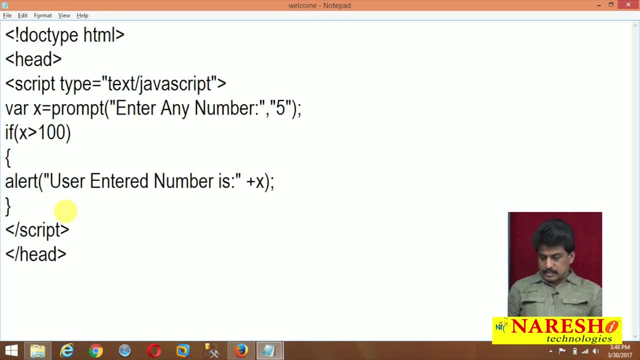 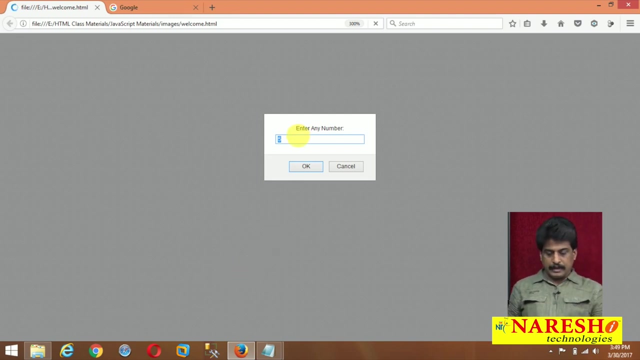 block. false means, else block. Come to else: environment Else alert. very basic programming Alert: user entered, Entered number is User. entered number is plus. Now I am giving it b for more understanding. Nothing is there. Come back. Yes, for example, I entered 5.. I am leaving like that, only Otherwise. 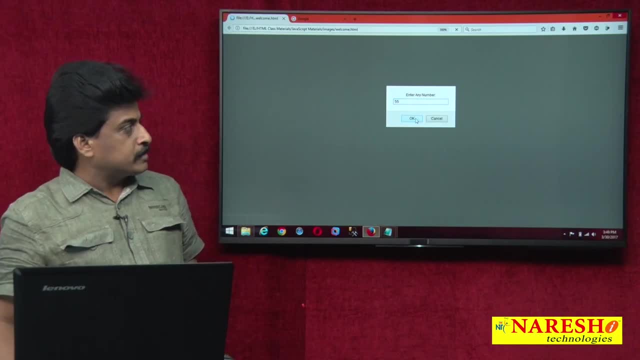 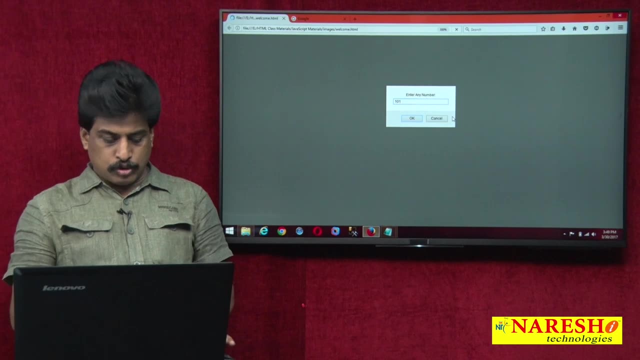 55,. no issue Greater than or less than Less than Else part will be executed. So I am giving it b Small. Now, for example, I am entering this 102, for example. It is a greater than So. 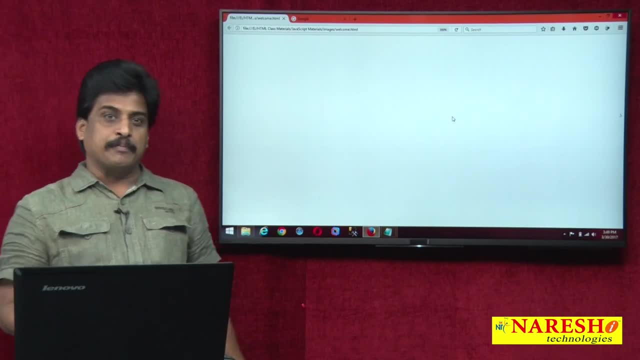 executing big Means if equal. what happened? That is a doubt. Else, if will write What is there. So now we are checking Greater or less than Now equal to purpose. Come to else if Now, for example, if you are coming to else, if block, Okay. So if you are coming. 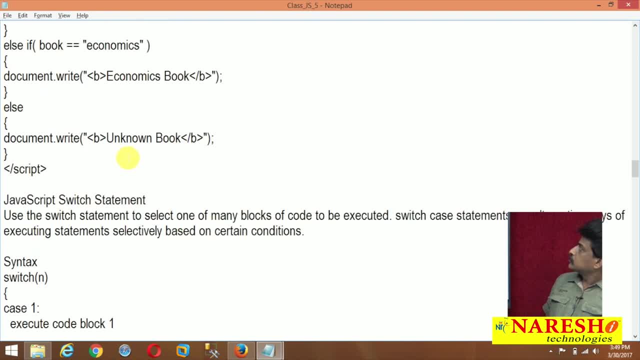 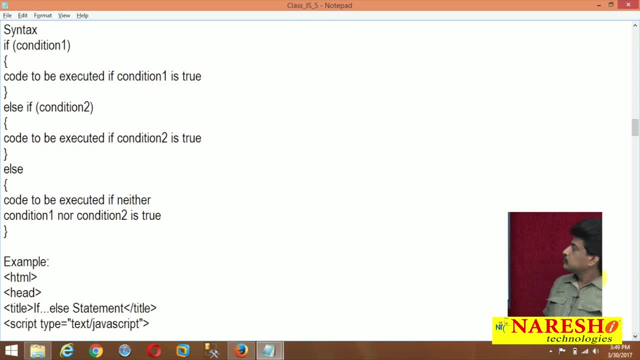 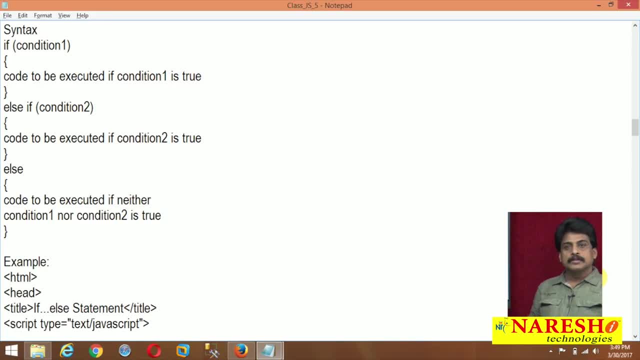 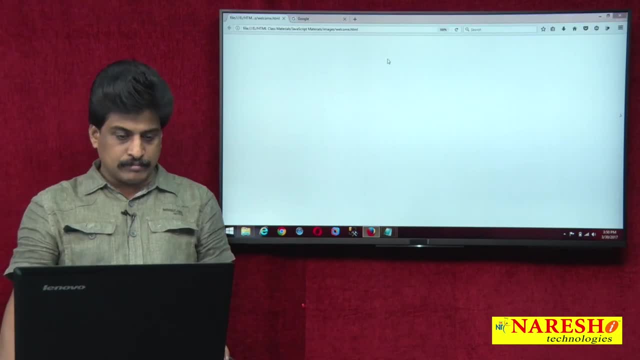 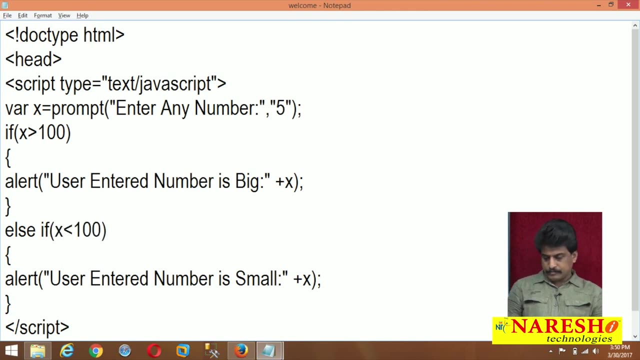 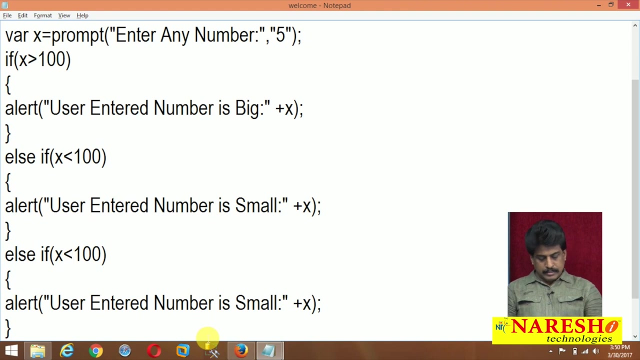 and the related blocks. Now in this syntax any one block of statements get executed. Definitely come down. We can view Whilst: if x less than 100, correct, Now the same else. if I want to take copy paste: x equal to 100 number is equal, else alert invalid input right refresh. 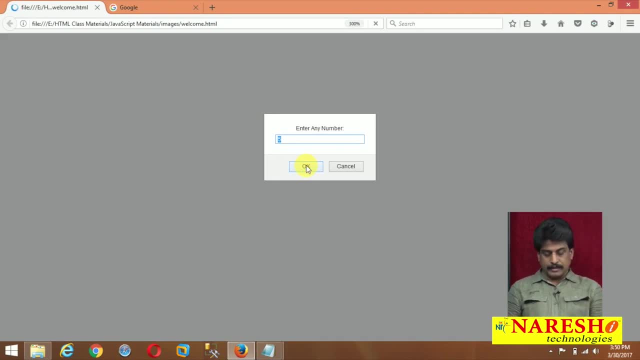 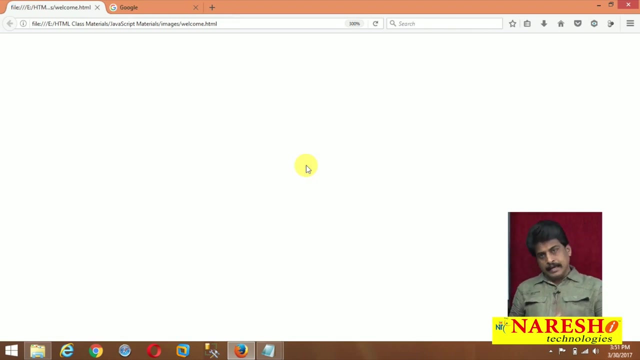 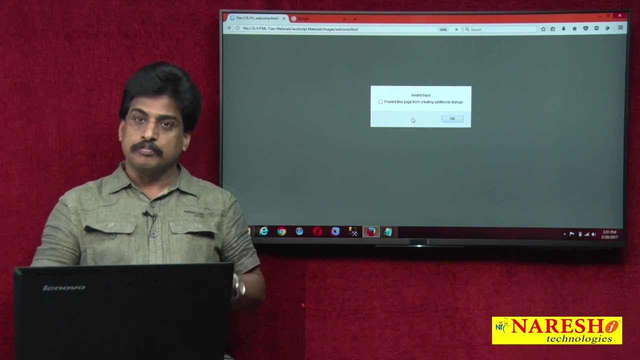 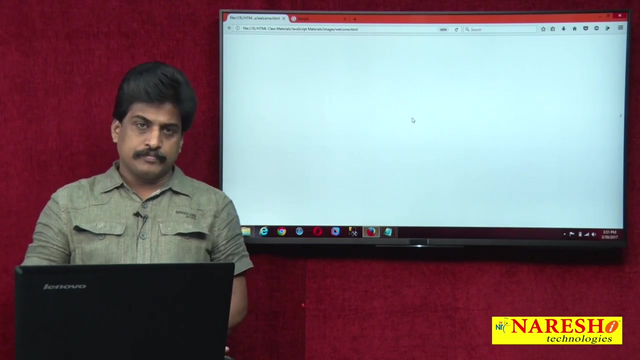 that. first one: I am entering 1, 0, 1, greater. you know already that yes. second, I am entering 100, equal, perfectly. observe third one: I am entering less, 55, small means greater, less equal. for example, I am entering Raju, invalid input, so perfectly. every condition checking and coming out. now we can view switch, same it. 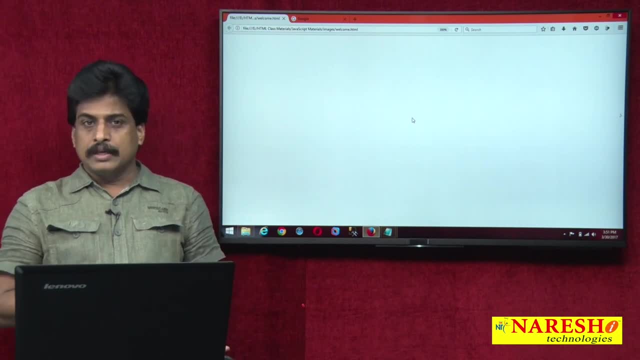 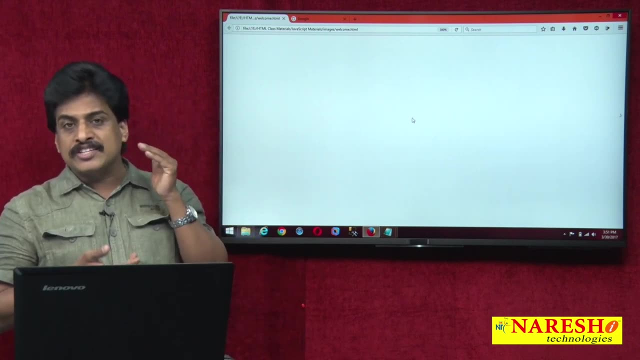 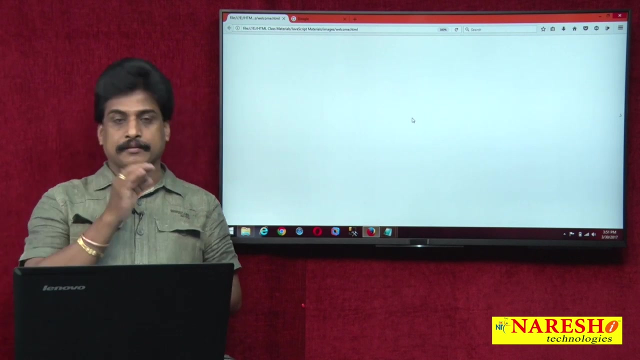 get executes any one block of statements. then generally, what is a big difference between LC, fun switch? switch is predefined structure. that is a reason compared to if switch performance always better predefined in the sense switch variable case break in between statements. what is the syntax of that? come to? 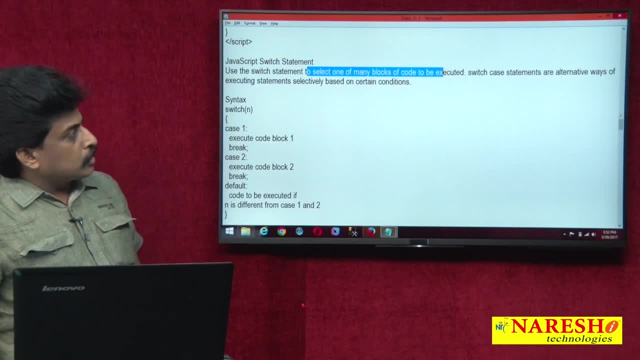 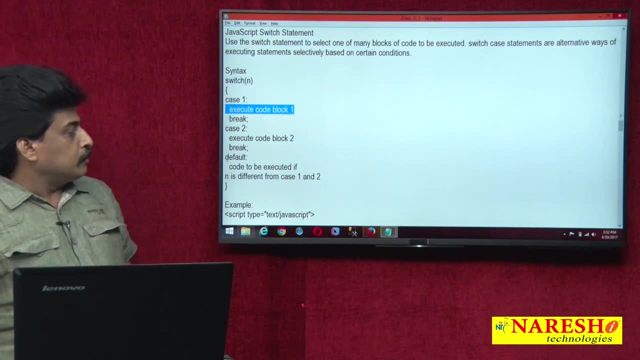 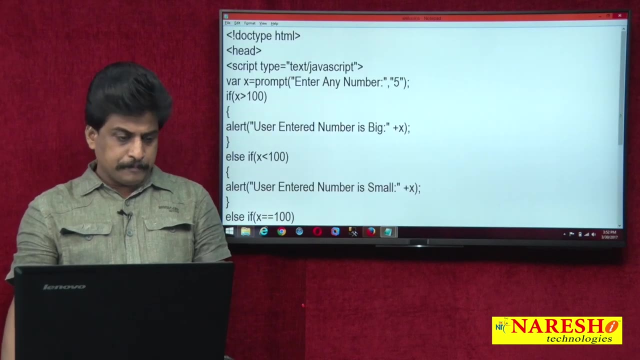 practically we can view switch: any one block of statements get executed. switch variable case, break in between the block and default also existed, same like our C programming language. now we can view that practically. for example, if I want to do a block of statements, I can do a block of statements. 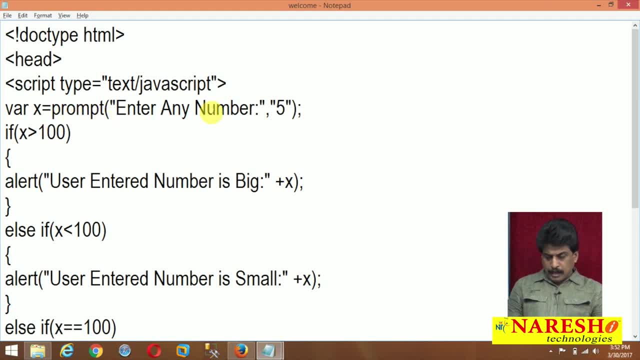 this like a example. now I am giving prompt any course name by default course. I am selecting HTML, if course equal to, if course equal to start HTML file. of course score will be the first of all start when we are not using first step left to 2.5, which is correct. our first step alonghan method, decoding m1, and I call our step off ger the first step. and, for example, instead of format keyword, a format field we are going to use: parent leaves Memphis. so for example, I: how to shovel that type code that should beайт Korean alphabet or kimono root, then G, strawberry, those letters in it, of course, and 사용h as�� fish income methodATLB. how we key NCTZE X is excited Huh. 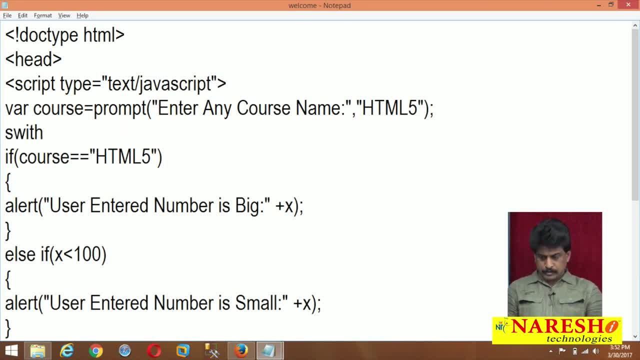 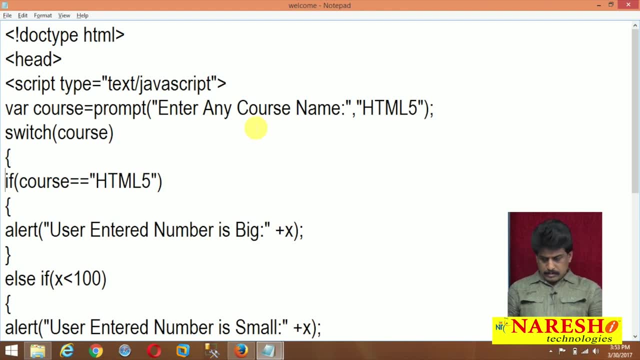 what just about taking the SQL Strips step is is like if you want to do it as step first, you Okay, directly switch. only I will show you Switch. what is that course Once that existed. now I am writing here case and I am going to show you here HTML5. 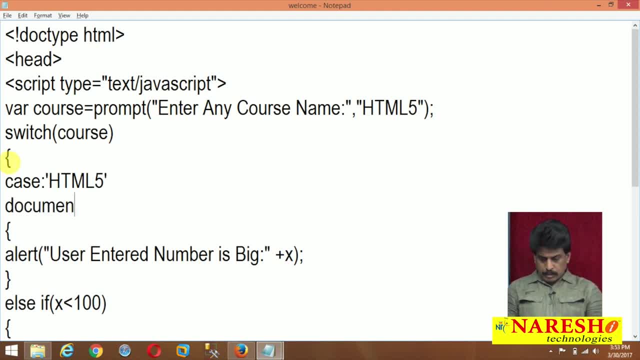 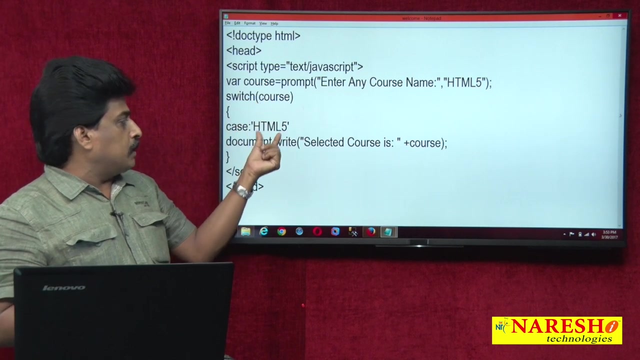 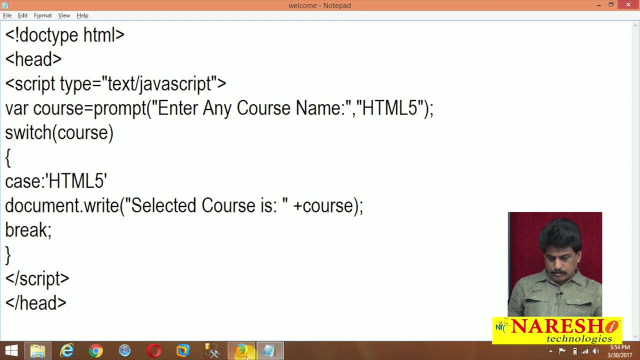 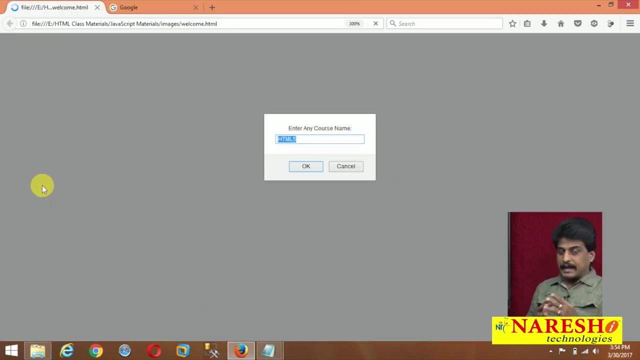 So once I am going to documentwrite, selected course is symbolized, for example, plus course. Now that one closed, Let me remove the remaining part, Course variable. I am reading that case: HTML5 documentwrite and syntax wise break. Now come back to your browser Refresh. So it is not asking that what is the case you actually selected Because syntax wise, we need this like this, Every syntactical rule correctly. we need to follow. 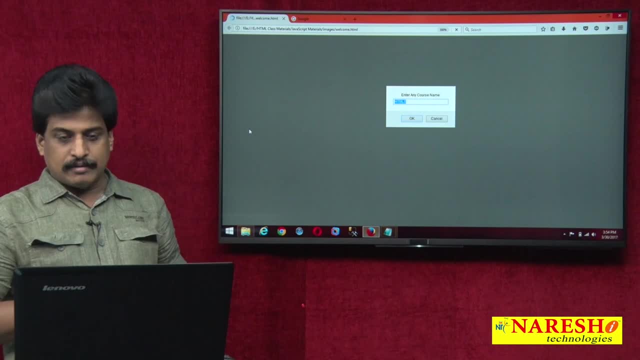 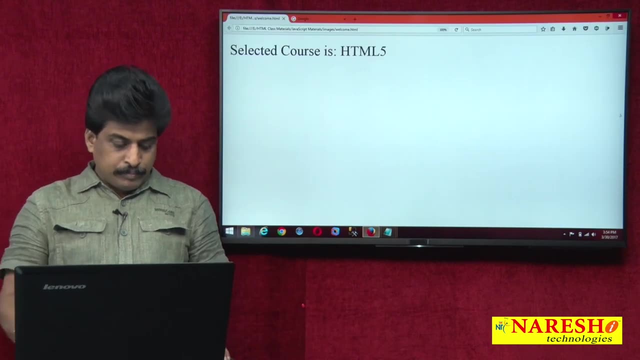 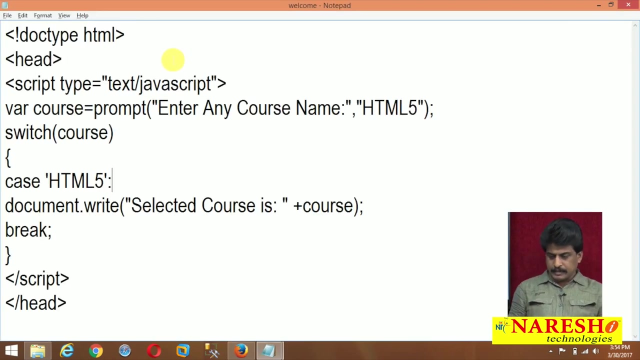 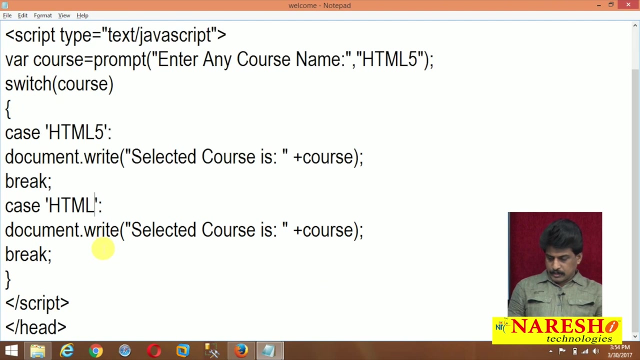 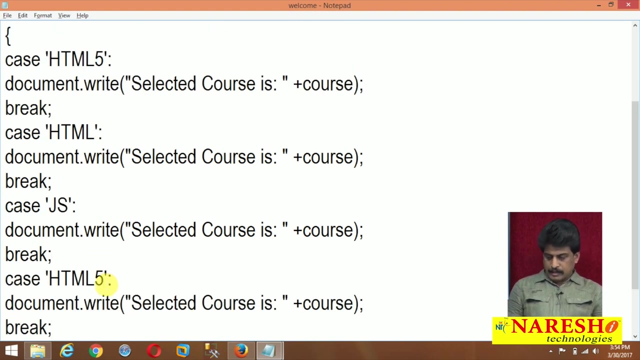 So the colon we need to end last asking, for example, by default, HTML5 is there. If I clicked you are, selected course is HTML5.. For example, HTML JavaScript. I entered for example JavaScript. is not there, Blank page will be displayed. Let me write the program Now case: I am taking next one, For example, HTML, Good, And next one. For example, I am taking JS. Next one, Angular JS.